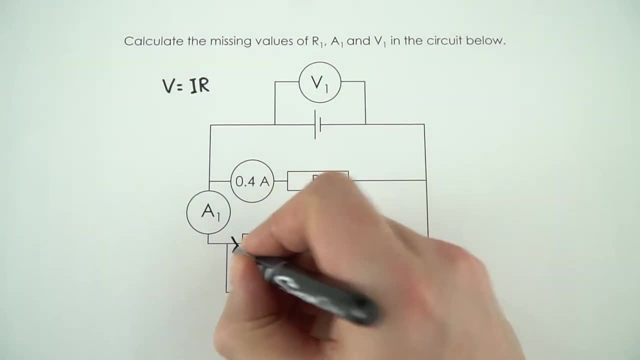 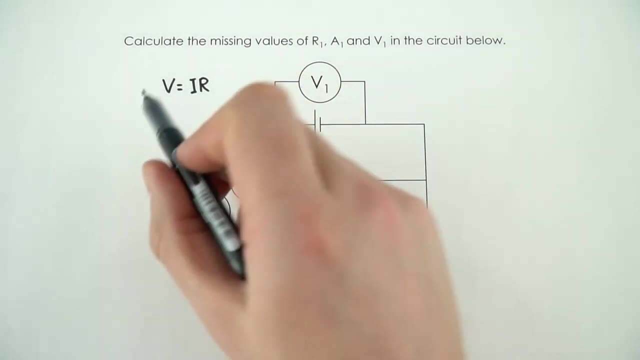 circuit, you have the same current everywhere. if we work out the current through this, that also tells us the current through this resistor and the current through that amateur. So I'm going to rearrange this to say that R1 is equal to I times R1, and I'm going to work. 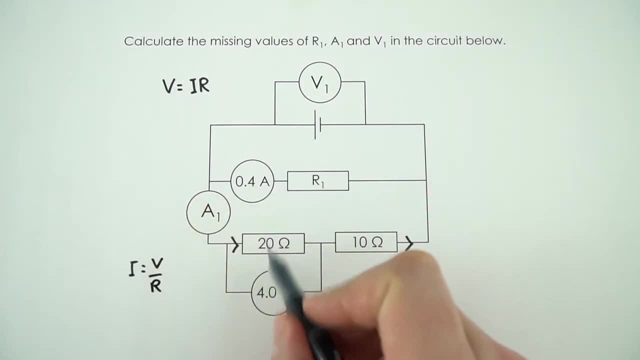 out, the value of I is equal to V divided by R. We know here that the value of V is equal to 4.0, and the value of R is equal to 20.. So 4 divided by 20 is the same as 1 divided. 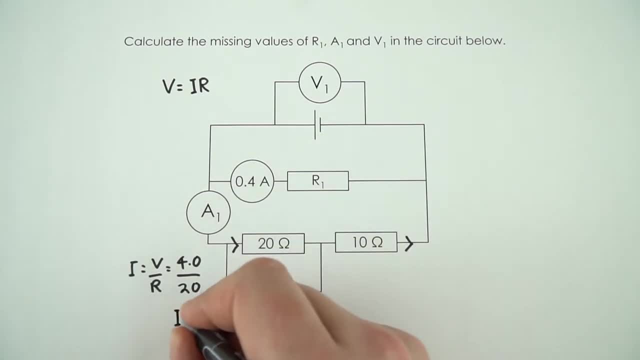 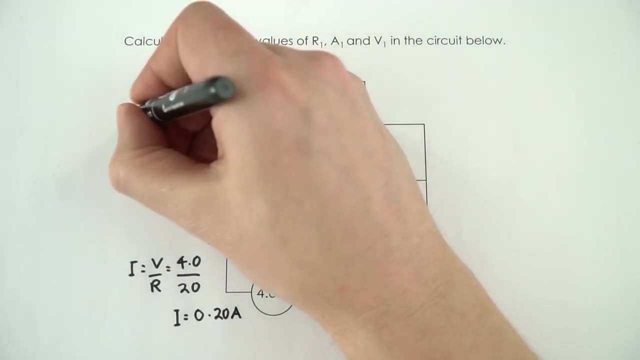 by 5, and that's just a fifth. So that means the current here is going to be equal to 0.20 amps. So what that means is our value for ammeter 1 is equal to 0.20 amps. So that's. 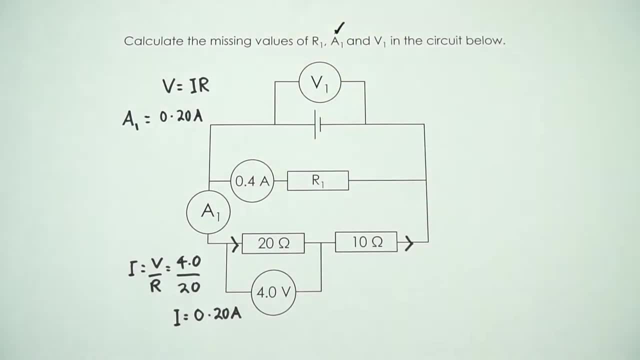 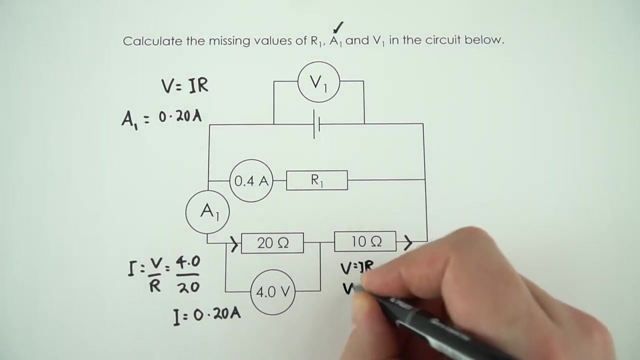 the first bit of information. Okay, what next? Well, we know the current through this resistor now, because we've just worked it out there as 0.20 amps. So what we can then do is look at the potential difference across this. So we can say that V is equal to IR and that means the value of V is going. 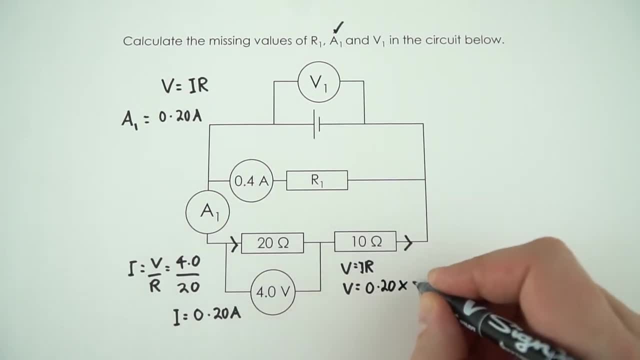 to be equal to the current 0.20, times the resistance of 10,, and that means the potential difference across this component is 0.2 times 10,, which is just 2.0 volts. Okay, now, we're not asked to find this in the question, but it's a useful piece of information. 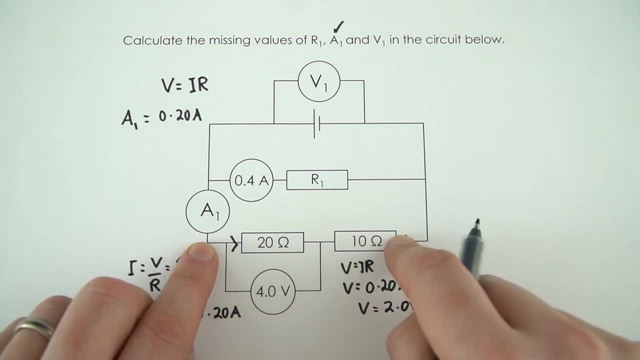 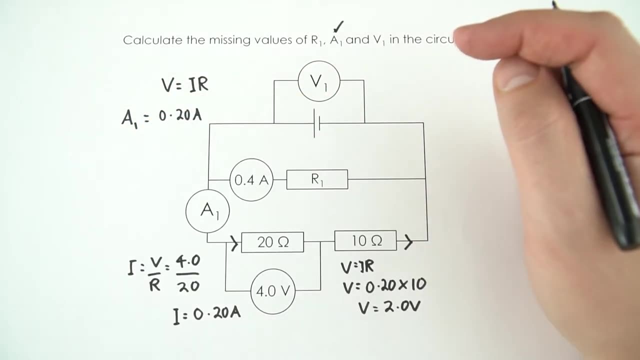 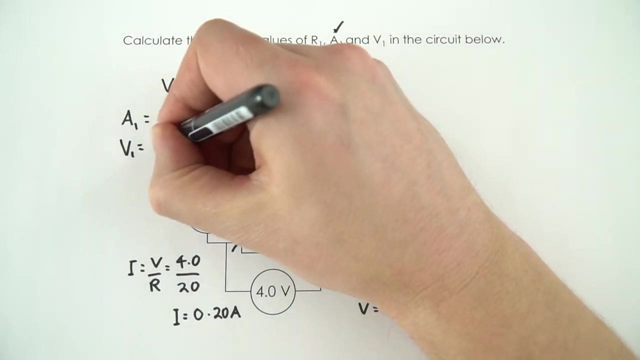 because if we know the potential difference across this and the potential difference across this, this must equal the potential difference across this, because the potential difference at any loop in the circuit is going to be the same as the source. So that means the value of V1 is going to be equal to 4.0 plus 2.0, which is equal to 6.0 volts. Okay, 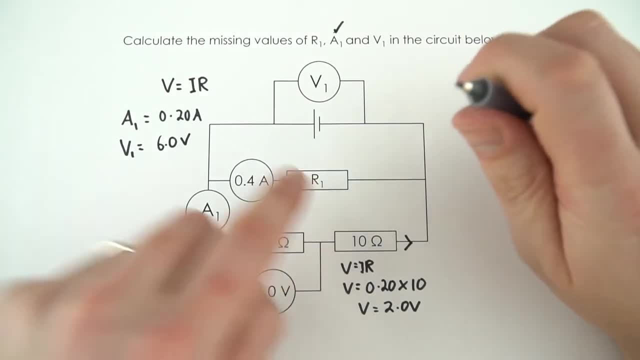 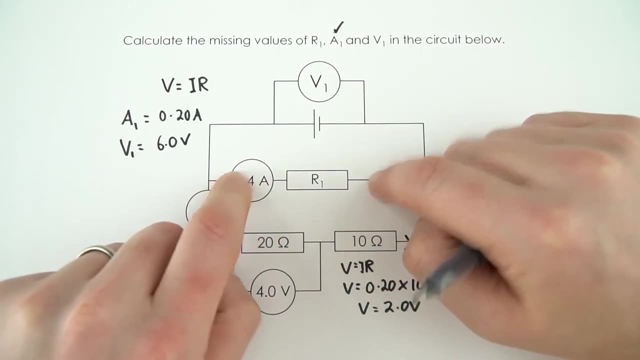 and now the final thing we need to work out is the value of this resistance. So we're going to look at this resistance. So because we know that that's 6 volts, this must also be 6 volts across this resistor. And again I might kind of sound like I'm saying the. 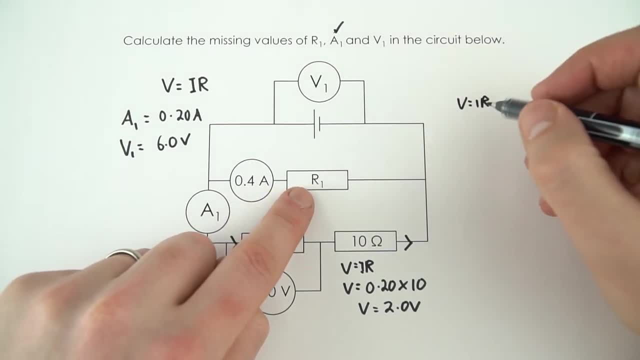 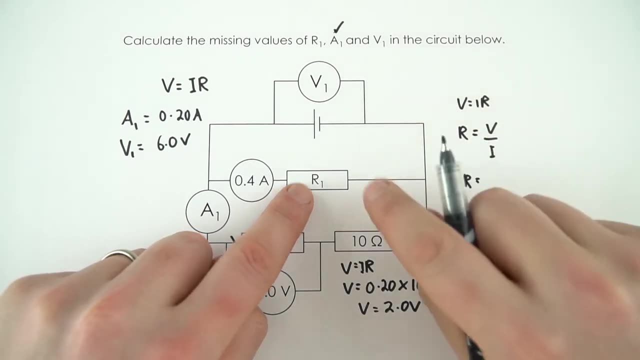 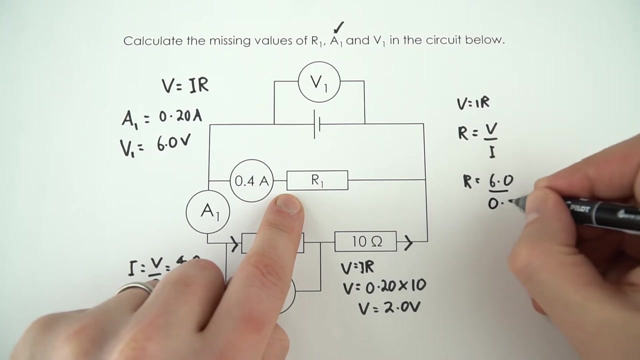 same thing, but V equals I times R Now across this resistor. we don't know the resistance, so R is equal to V divided by I. So the resistance here is going to be equal to the potential difference, which is 6.0, that we worked out earlier. We divide that by 0.4, which is the